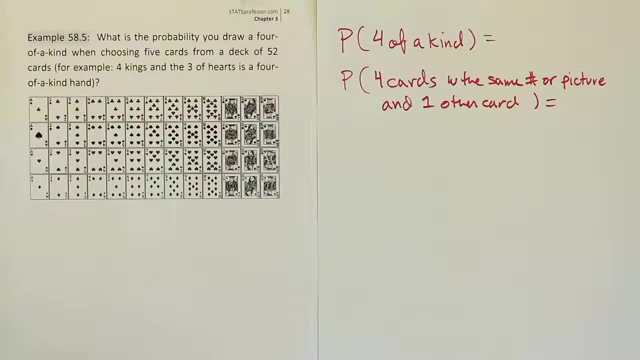 I don't want to go into a whole proof of to understand why this is true. We could do that but it would take a lot of time. And remember these problems are mainly set up for us to just quickly understand how to do example problems. 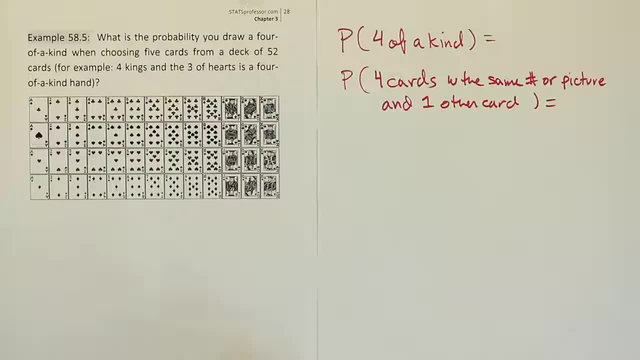 So I don't want to go too heavily into theory here. But if you were to create, for example, five fractions that represent the five selections of cards and you tried to solve the problem that way, you would get it wrong. And the reason why you would get it wrong is mainly because when you do that, you allow for the possibility that the same five 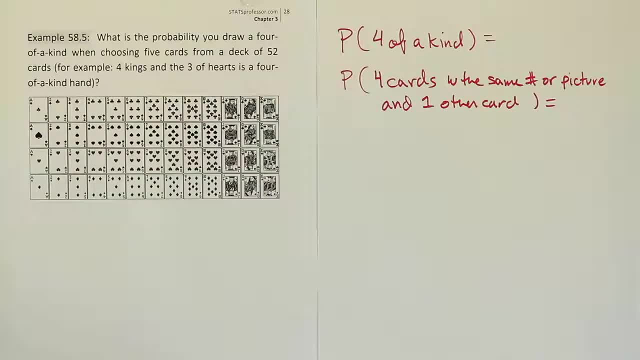 Card hand scrambled up in different orders to be counted separately as if they're different hands. So if we try that approach, it's not going to work. So what we have to do instead is to use combinations, because with cards, as long as you have the same five cards in your hand, it counts as the same hand. 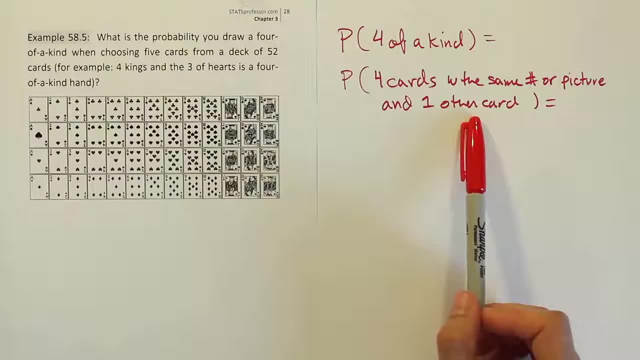 Right. It doesn't matter how many different ways you permutate or scramble up five cards, It's still the same hand if it consists of the same five cards. All the different orderings of those five cards should only be counted once, So that means we should be using combinations to solve this. 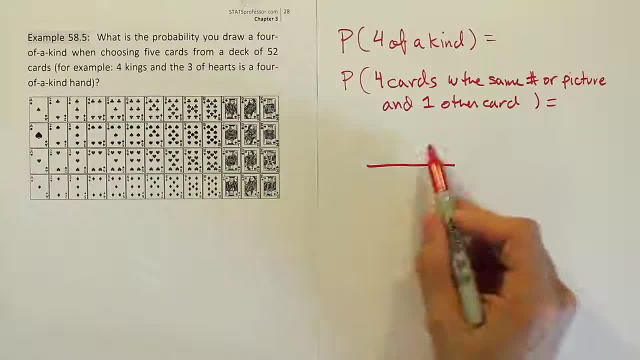 So we're actually going to have two combinations, or actually more than two combinations, But the top and the bottom of the fraction here is going to be filled with combination symbols. So let's start with the top part. It would be the number of four. four of a kind hands. 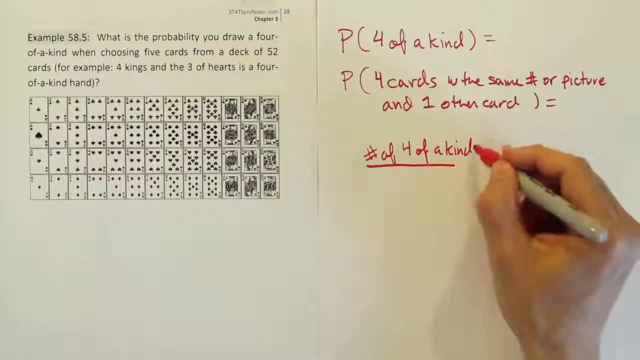 Right Four of a kind hands- And again that's very difficult to figure out Divided by the Total number of five card hands. So we've already looked at this bottom part in another problem. We can do that pretty easily then. 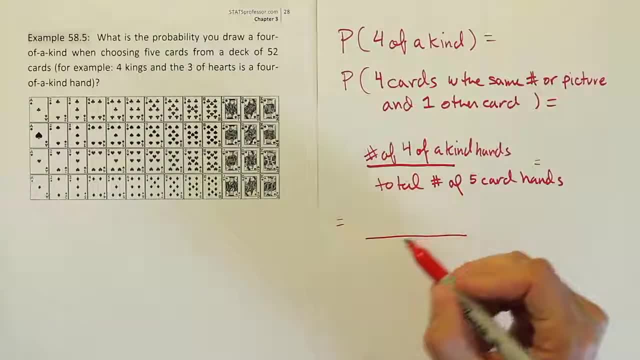 For the bottom part of the problem, that's pretty simple. Out of 52 cards we want to choose five cards. That's all the different five card hands that are possible. We actually saw in a previous example that was something like 2.6 million different possible five card hands. 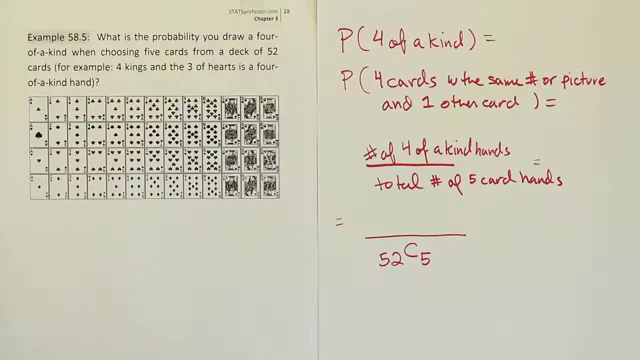 Now, how many of those card hands are actually four of a kind hands? You could literally list all the possible four of a kind hands. You could create a huge list of all those And when you were done, you know you would have the answer. 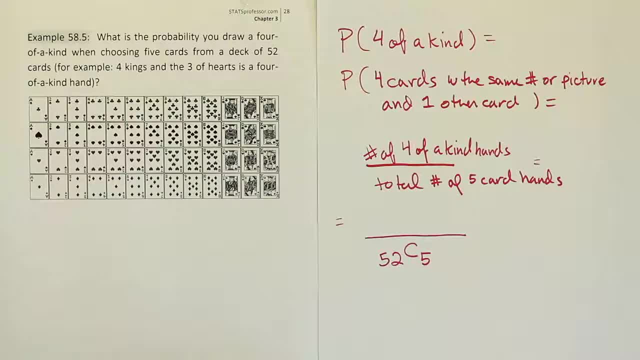 But that takes a long time. So to avoid having to do that, the brute force method I would call that- we're going to use combinations to do it, And the way it's going to work is we're going to think about: if you wanted to construct a four of a kind hand, how would you actually have to do that? 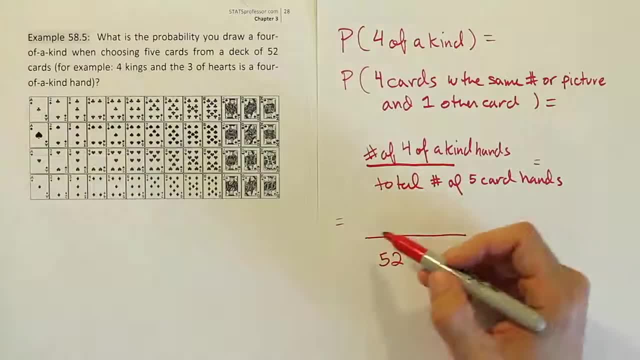 Well, the way it would be constructed would be as follows. You'd have to say: hey look, first thing I need to do is to figure out which you know card. I'm going to have four of a kind hands. So, for example, do I want the queen to be four queens or do I want four kings in the problem, right? 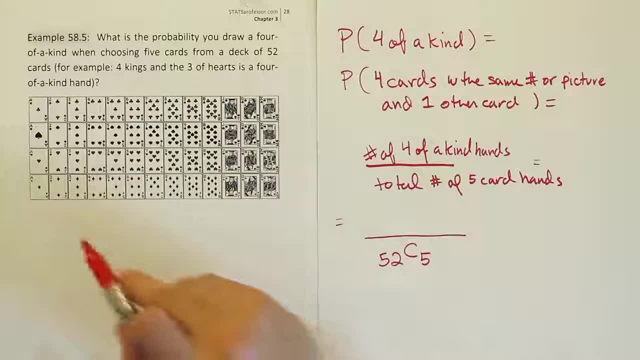 We'd have to figure that out. So, in other words, if you look at the number of possibilities, then we could pick any one of these cards to be the card that gets four of a kind with right. So, for example, out of the 13 different possible cards that are there, right? 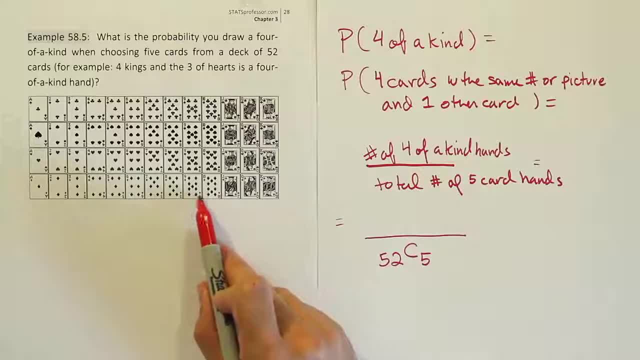 So, in other words, there's 1,, 2,, 3,, 4,, 5,, 6,, 7,, 8,, 9,, 10,, 11,, 12,, 13 different possible cards that we could choose. 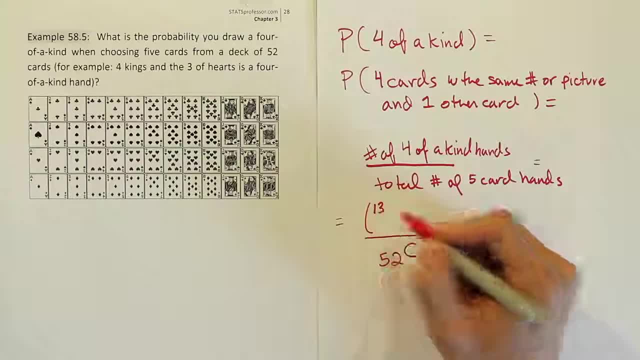 So I'm going to say, out of 13 cards, right, I want to choose exactly one of them to be the card that's going to have four of them, right? So four cards of the same number or picture. I'm going to pick which card that's going to be. 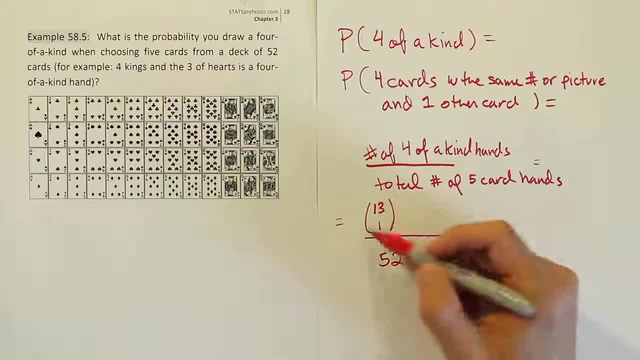 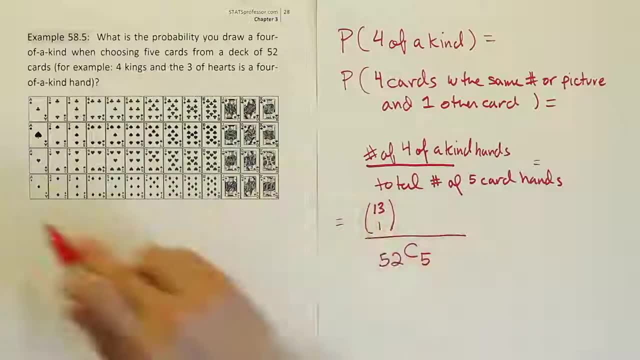 This notation is the same as the combination notation, right? It's just a little more concise, so I don't have to keep putting the C over and over again. This is 13. choose 1.. Alright, so out of the 13 cards I could pick, I'm going to choose one of them to be the card that I take 4 from. 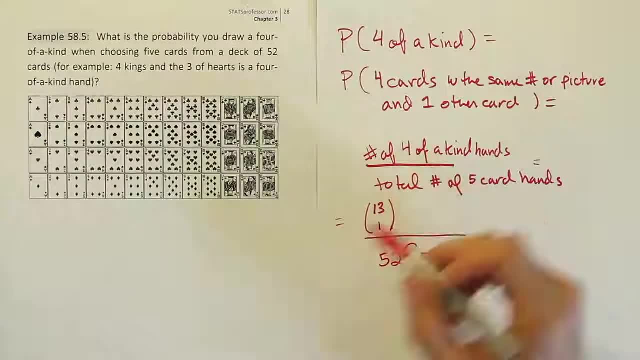 Now, technically, if you want to be precise, once I've picked which one, let's say I decide I want 4 aces, So I'm going to pick my aces. That's when I do the 13, choose 1.. 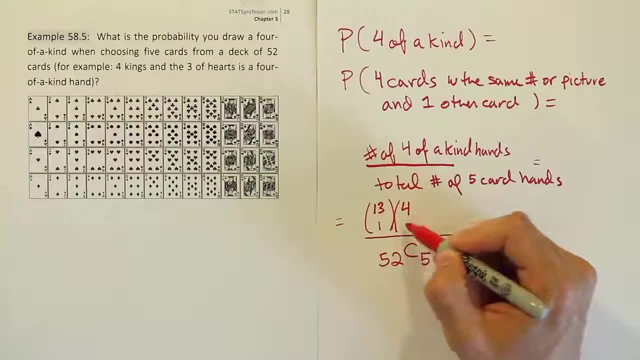 I've chosen aces. Now, out of the 4 aces, I have to choose all 4 of them. This part of the problem could actually be left out, because there's only one way to do that right. If you choose all 4, there's just one way for that to happen. 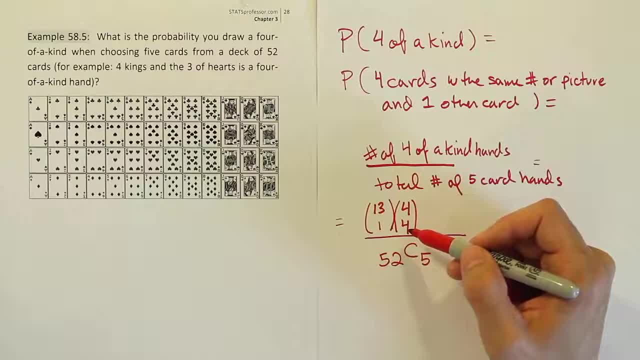 If you work out 4, choose 4, it does give you 1.. But I just want you to get in the habit of thinking properly here. First, we're going to choose which card is going to be in the 4 of a card hand right. 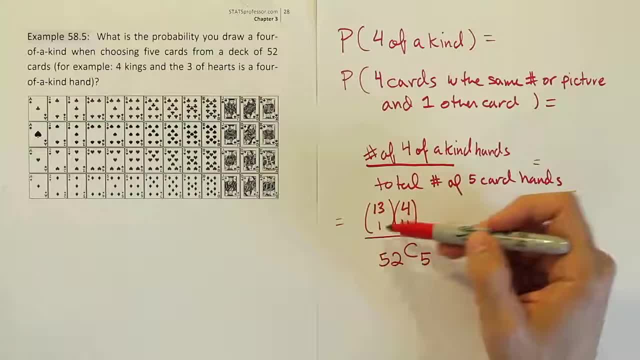 Okay, And then we're going to choose all of those cards. So now we have all 4 aces, right? So we're almost done constructing our 4 of a kind hand. And it's completely general right, Because this one card could be aces, or it could be kings, or it could be queens, right? 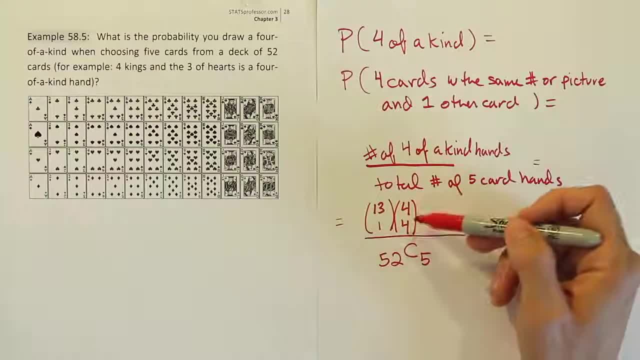 Whatever, Whatever card I choose here, I take all 4 of them. Now we're almost done. We have 4 of our 5 cards, But we have to pick the leftover card And there's 2 ways to think about this. 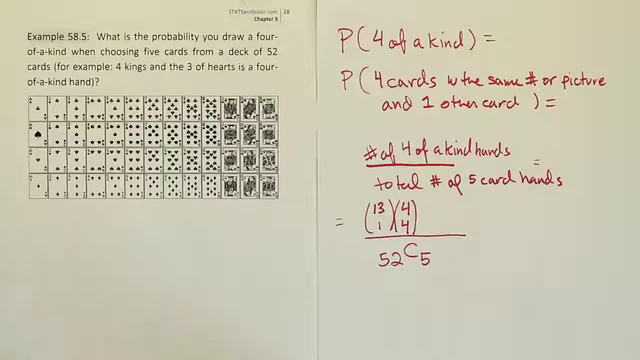 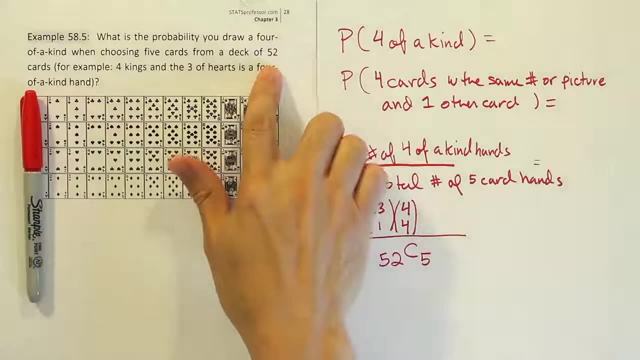 One way is to say: well, gee, how many cards are left in the deck? Let's say: I chose all of these cards right, So I've gotten all of those. Well, how many cards are left? Well, there's 52 cards originally. 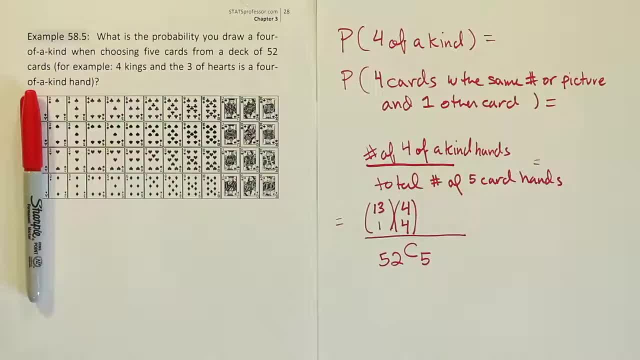 So there's actually only what 48 cards left, And then out of 48 cards I have to choose one of them. Any card will do So 48 choose 1 would work. That's one way to do the problem. 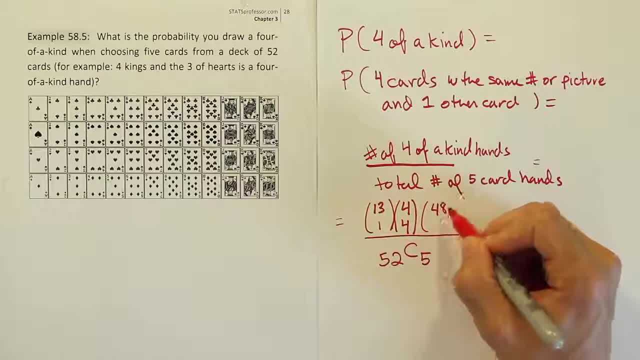 So you could say that and finish it up that way: Out of the 48 remaining cards, choose any one of them to be the fifth and final card, because it doesn't matter what card it is. Or the other way to do this is to say, hey, same thing, right. 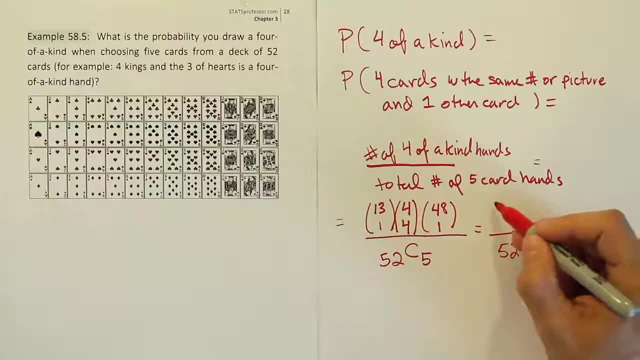 You know 52, choose 5.. You could say, hey, look, out of 13 possible cards, I choose the one card I'm going to have 4 of, And then I'll take all 4 of those cards, right. 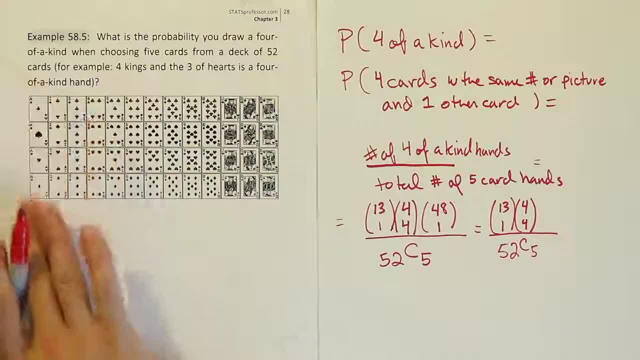 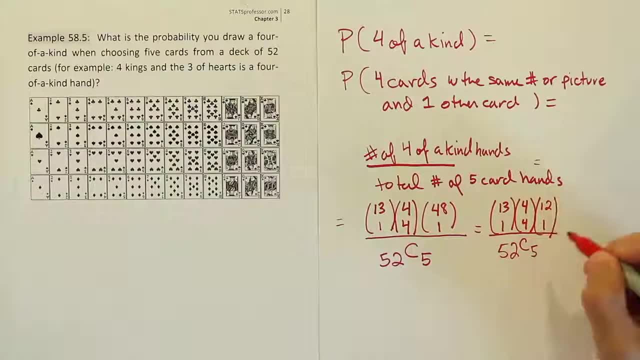 And then you could say something else. You could say: okay, well, I chose aces. let's say How many cards are left to choose from? Well, there are 12 different types of cards to choose from. I'll choose right one of those to be my leftover card source. 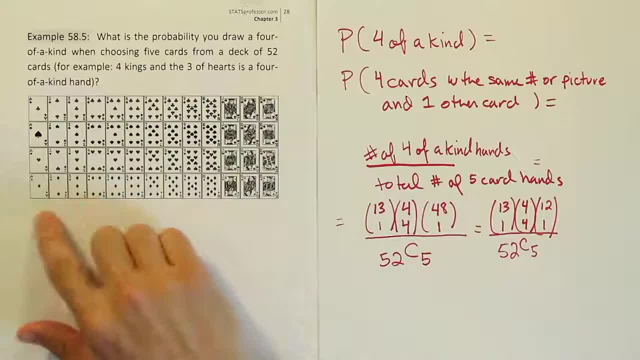 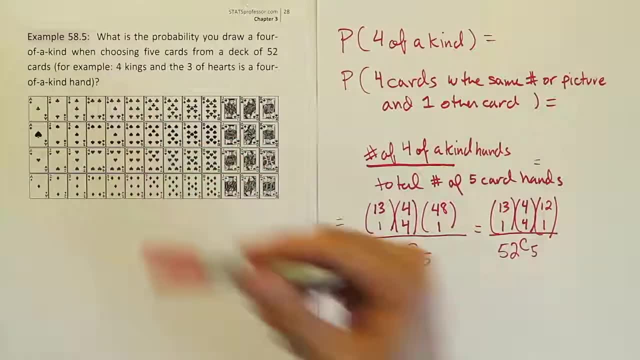 In other words. so my one extra card will come from maybe the 5s. So maybe I have 4 aces in one of the 5s. So I'll choose to choose from the 5s And then from the 5s. I have to pick which particular 5 I want to fill my hand with. 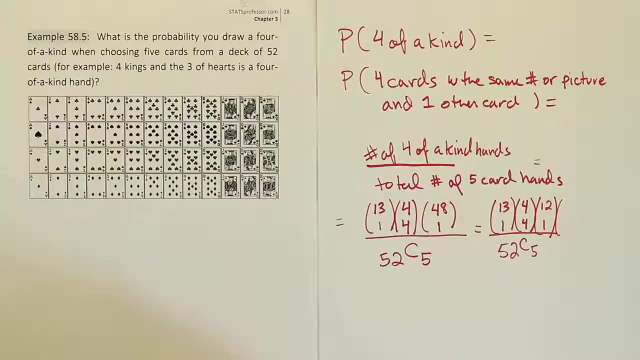 In other words, do I want it to be 4 aces and the 5 of clubs, or do I want it to be 4 aces and the 5 of spades, right, That sort of thing. So once I choose, 5s, right. so out of 12 remaining suits, I choose. 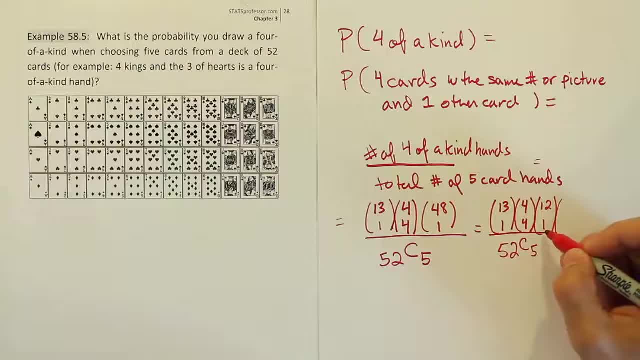 or 12 remaining cards to choose from. I choose the one you know set of 5s to work from. Then, among the 5s out of those 4 cards, I'm going to choose the one 5 that I want to use in my hand.